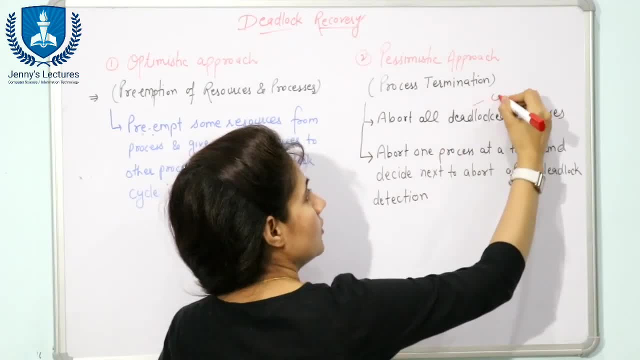 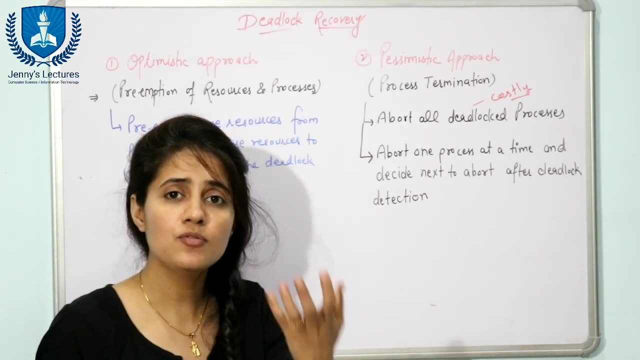 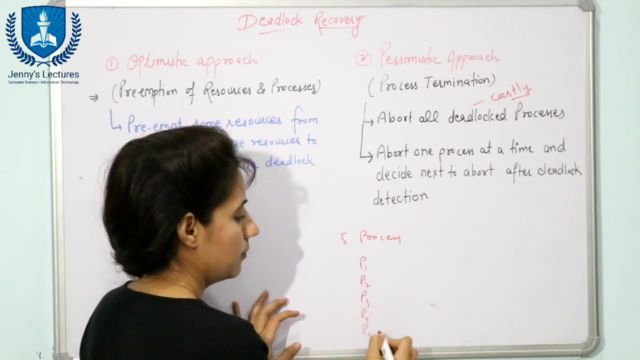 may be very costly. So the drawback of this case is what It is very costly method to abort all the processes. See, let us take one example. Maybe five processes are there which are in deadlocked state: P1, P2, P3, P4 and P5. 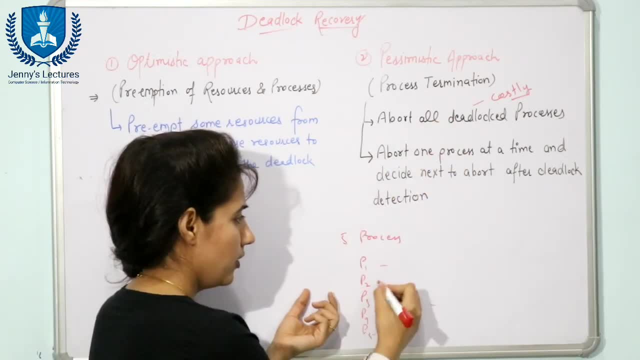 And essentially you can say: kill all the processes which are in deadlocked state. See costly in what sense? Maybe? suppose P1 and P2 has completed its execution up to 90%. Fine, suppose it 10%. This one is 10% and this one is 20%. 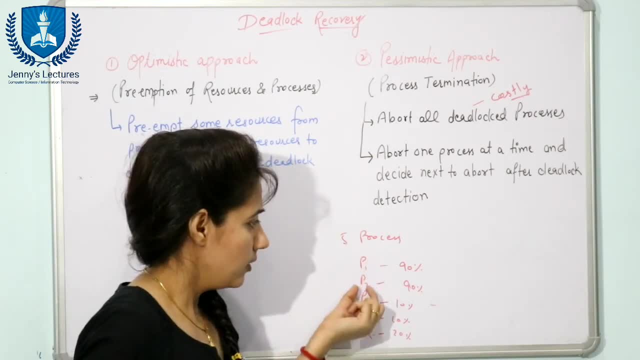 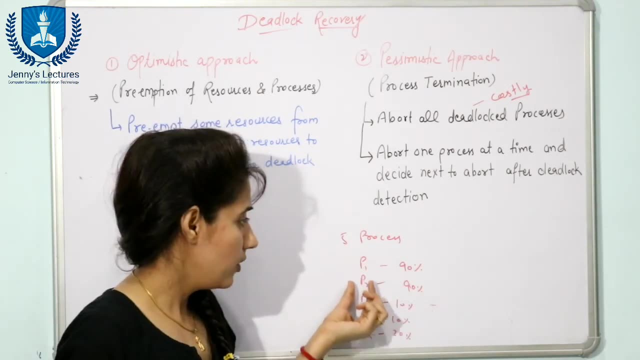 So see, when you'll abort all the processes, then the P1 and P2 will have to, then these processes will have to starts their execution from the starting only. But see, P1 and P2 has almost completed its execution, So it is not a good idea to abort. 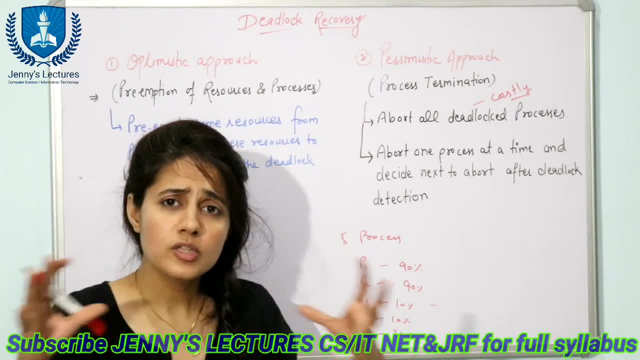 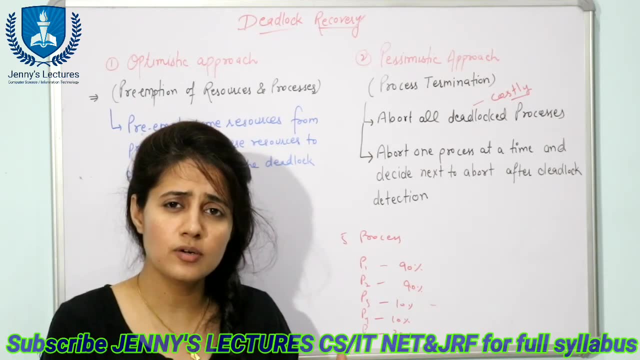 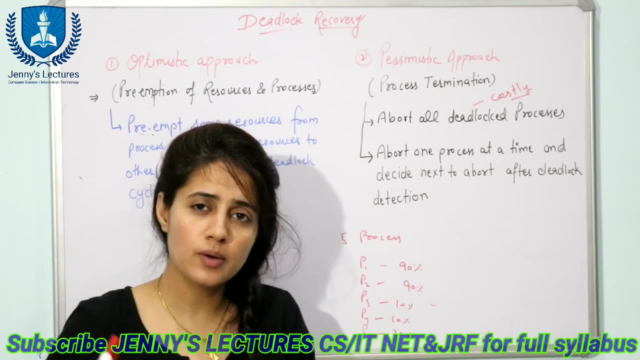 these processes. so it is not a good idea to about all the processes who are in deadlock state. why so? because maybe some processes may have executed, may have computed their work for a long time. fine, and when you'll about all the processes, then they'll have to recompute all the they have. they'll have to. 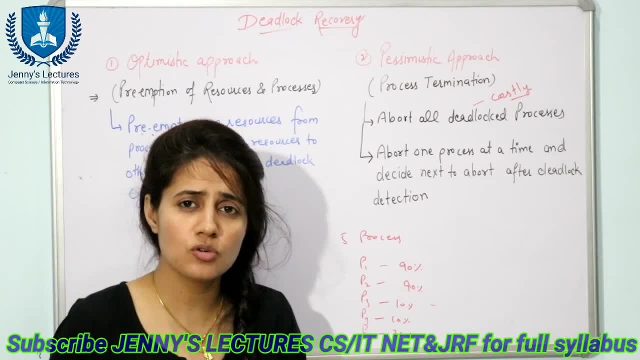 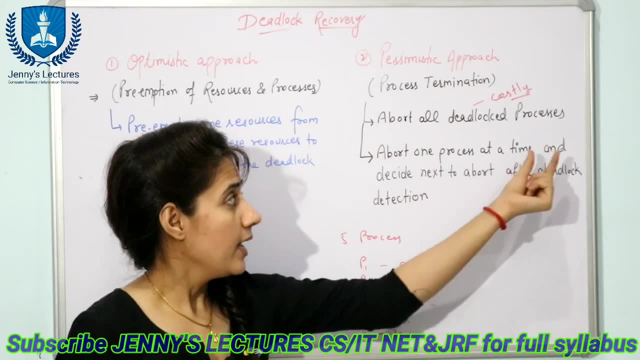 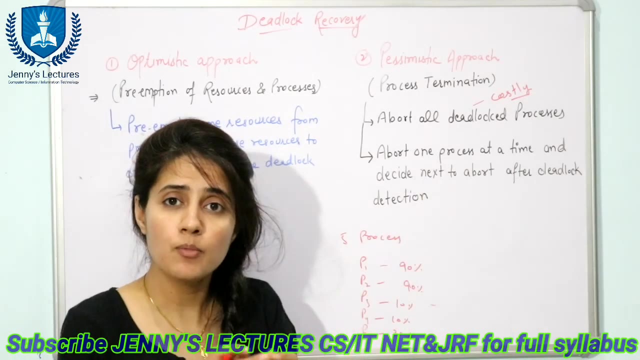 recompute all its calculation from starting. only so that is not a good idea, fine. so next thing is about one process at a time, fine, and then decide the next one. decide the next one. to abort after deadlock detection means about one process at a time, then apply, or you can say, invoke the deadlock detection. 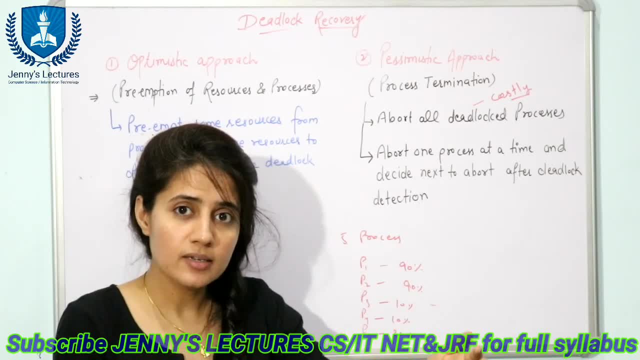 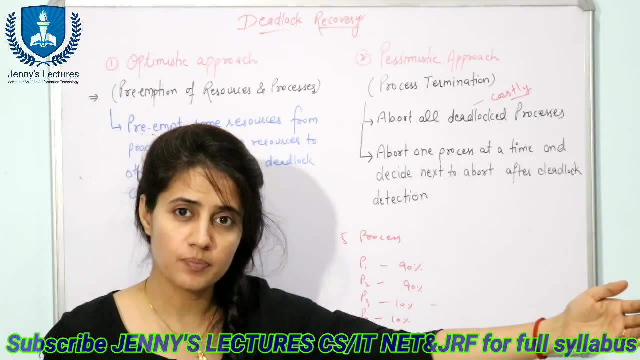 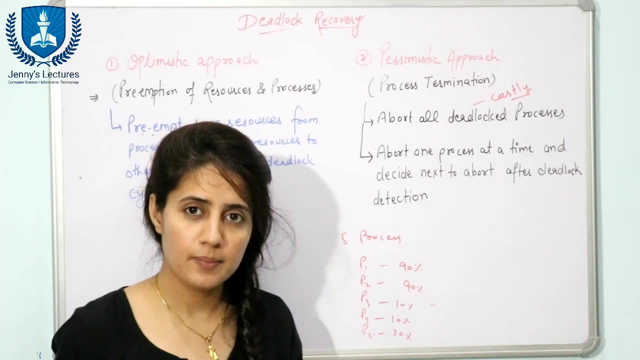 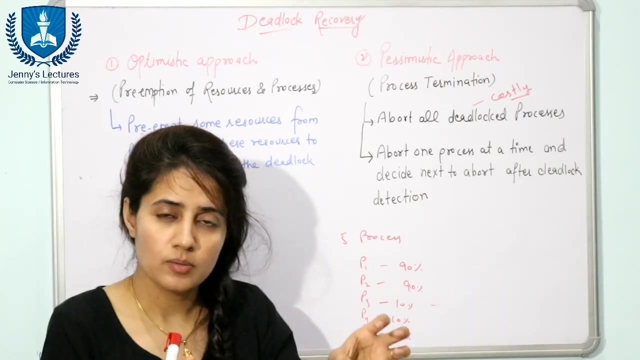 algorithm, if still detection cycle is there then, and then choose the next process to abort, then again invoke deadlock detection algorithm and keep repeating this step. and until what? until the deadlock cycle is eliminated. but see, see, drawback of this case is what: you are selecting one process and you are calling detection algorithm, again selecting. 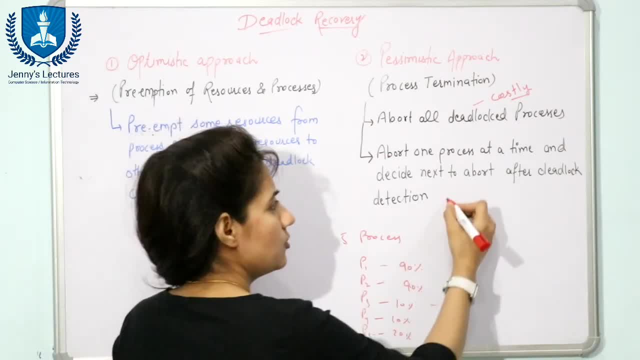 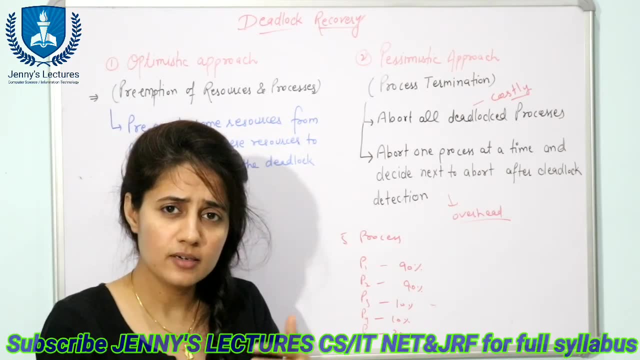 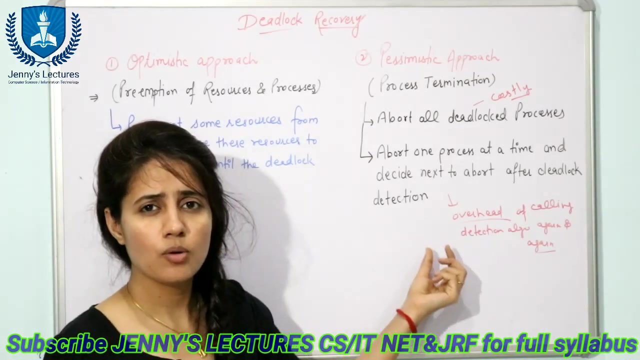 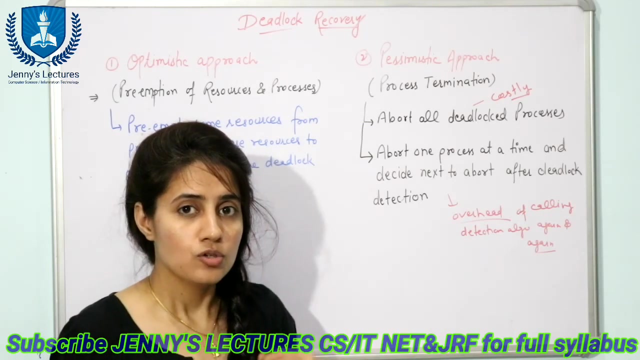 one process again calling detection algorithm. so this is basically a. it contains overhead of invoking the deadlock detection algorithm again and again after each, after killing of each process. so in this case you can say: the drawback is overhead of calling detection algorithm again and again after termination of each process. fine, so here here the funda is: we should terminate. that process, fine, we should terminate that process whose termination will cause minimum overhead and minimum cost to the system. now, how to? how to select that process whose termination will cause the minimum overhead and minimum cost to the system? there are many factors. basis on those factors, you can select to terminate a process and those factors are so. these are some. 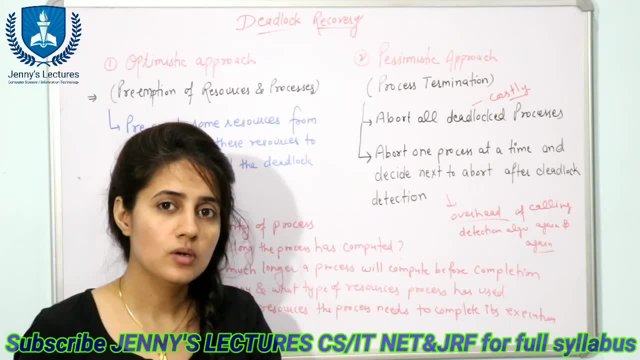 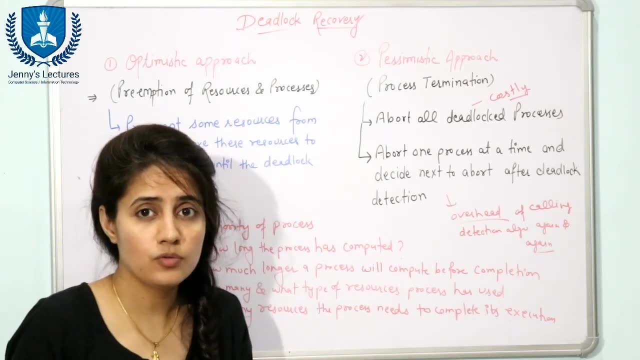 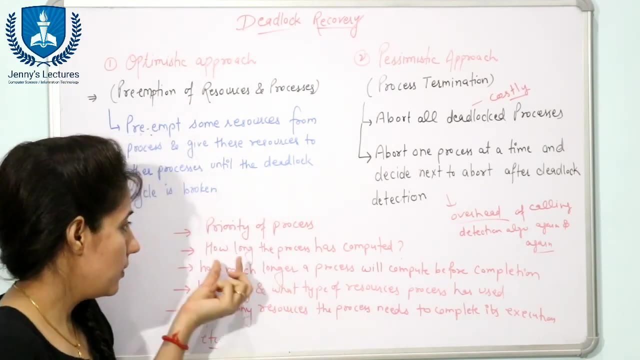 factors to be considered when we are selecting a process to kill. like what? what is the priority of the process? if process is having higher priority, then we, obviously we don't. we, we don't kill that process. we used to kill a process which is having lower priority- fine. next, next maybe, how long the 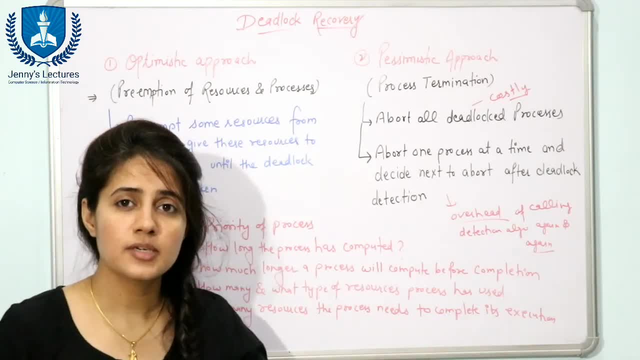 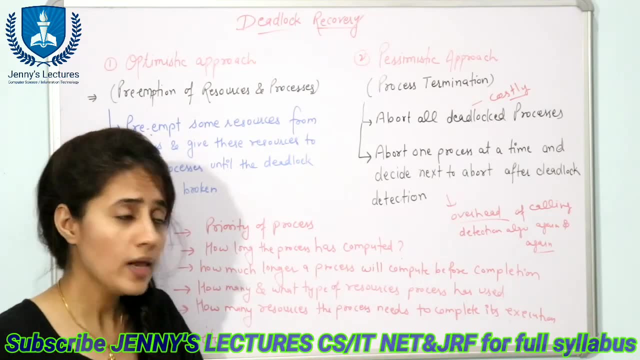 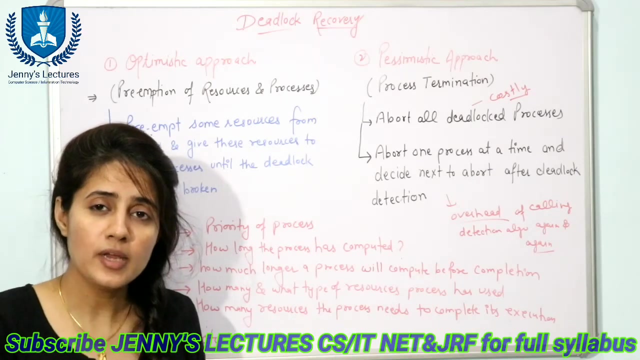 process has computed. maybe a process has completed its 90% execution, so it's better not to abort that process, fine. third thing may be how much longer a process will compute before execution, before completion: fine. next funda, maybe how many and what type of resources that process has used. 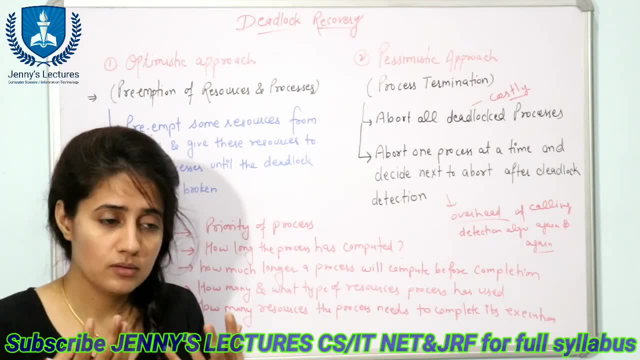 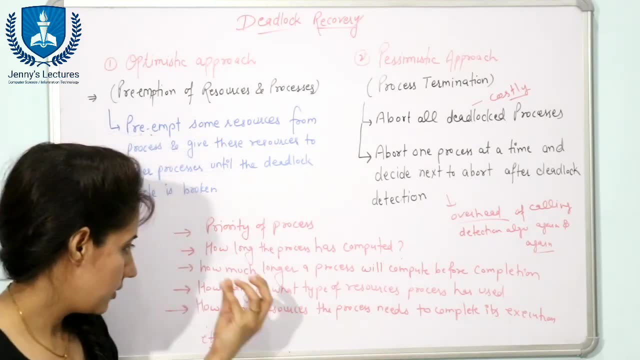 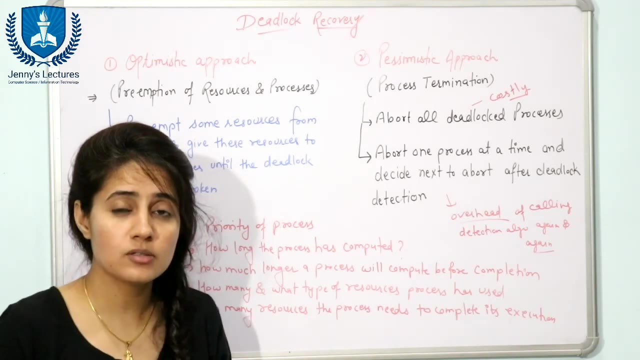 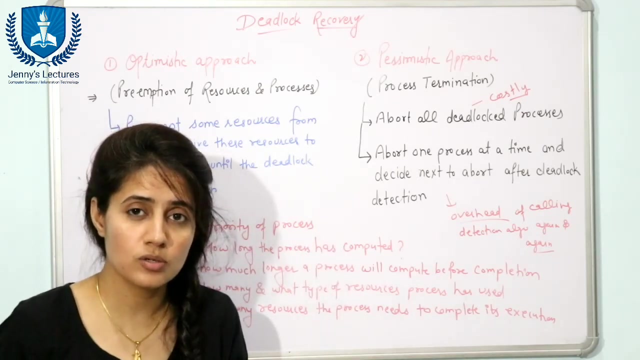 fine. Next thing, maybe, whether the process is interactive process or a batch process. next thing which is to be considered is how many resources the process needs to complete its execution. fine, maybe a process needs one more source to complete its execution, or maybe you another process needs ten more resources for its execution, so it's better. 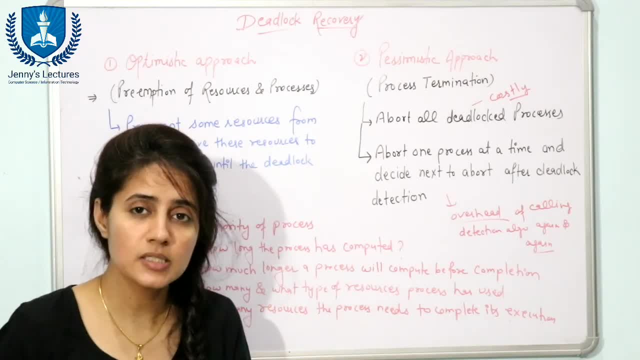 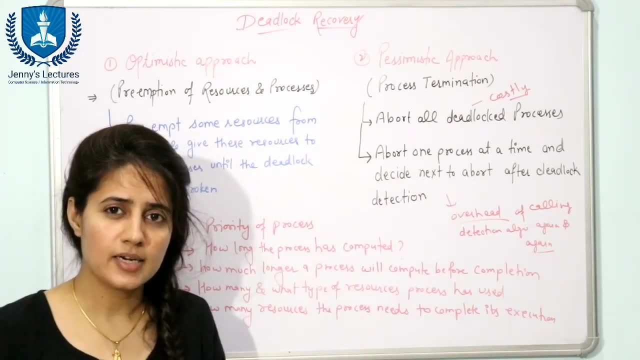 to about that process which needs ten resources for completing its execution, rather than the process which needs just one more resources to be used. need ten more resources? for Premierか, only one resource. These are some factors to be considered when a system is selecting a process to 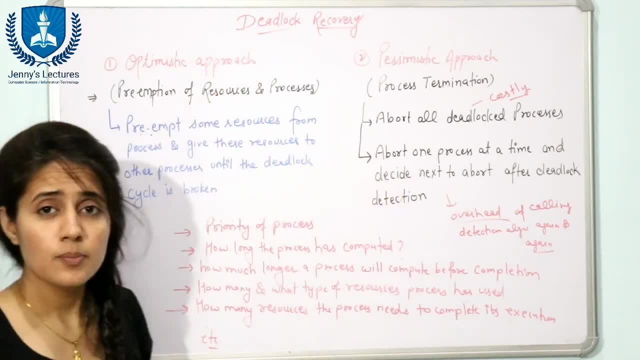 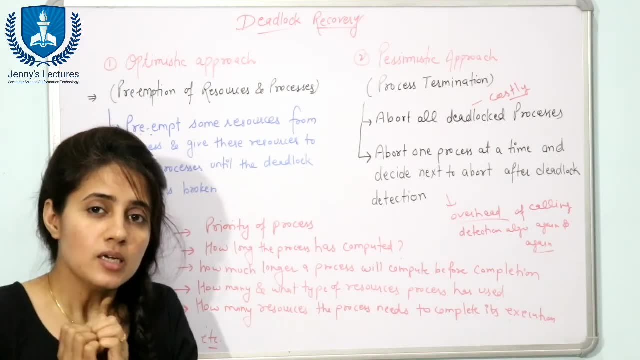 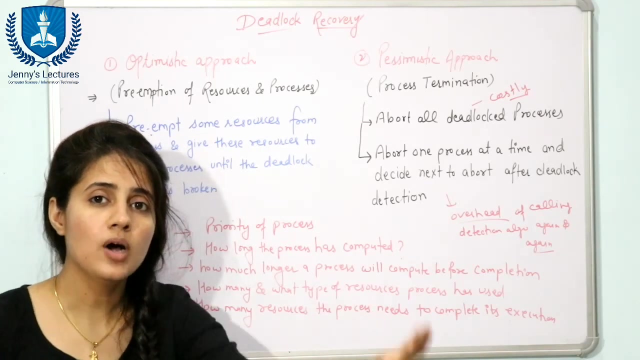 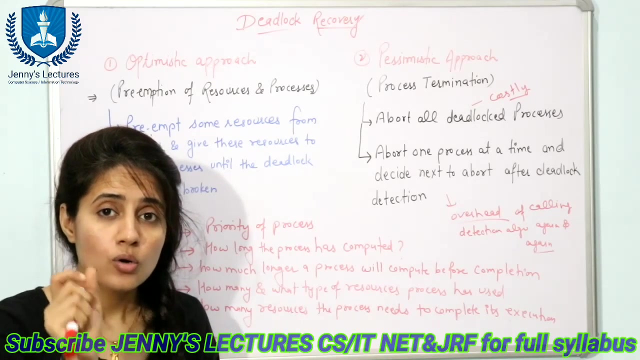 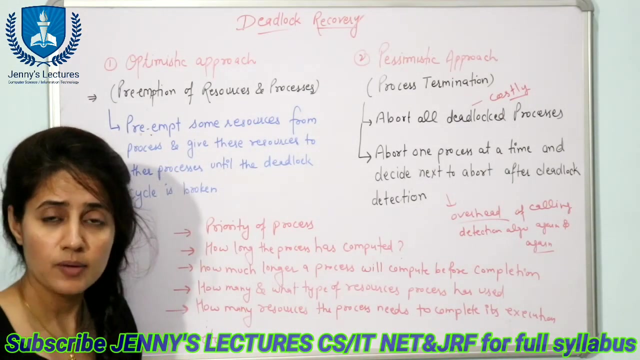 kill, Fine. Now the optimistic approach is: this approach is preemption of resources and processes- Fine. In this case, some resources would be forcefully preempted from any process and that resources would be given to another process so that the another process can complete its execution, Fine. Now, here here, the question is: see: preempt some resources from process, Fine. 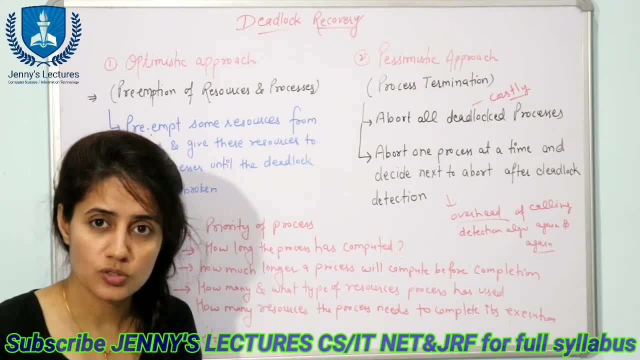 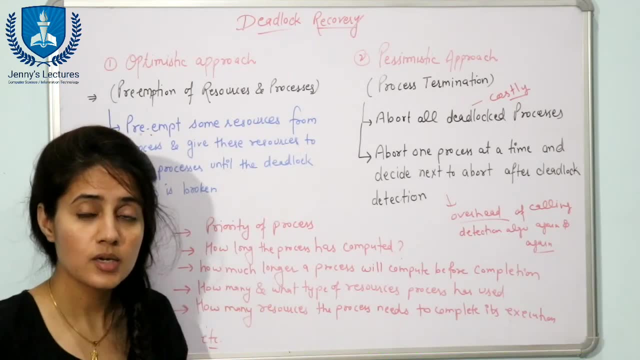 But the question is from which process you will preempt the resources. So so, when, when a system is implementing this kind of approach- preemption of resources and processes- then basically it needs to handle three problems. So these three problems are: selecting a victim, rollback and starvation. 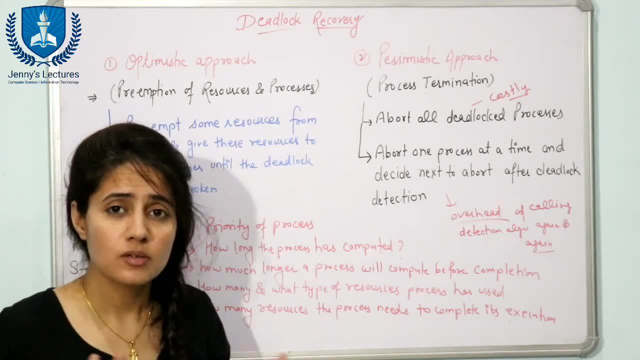 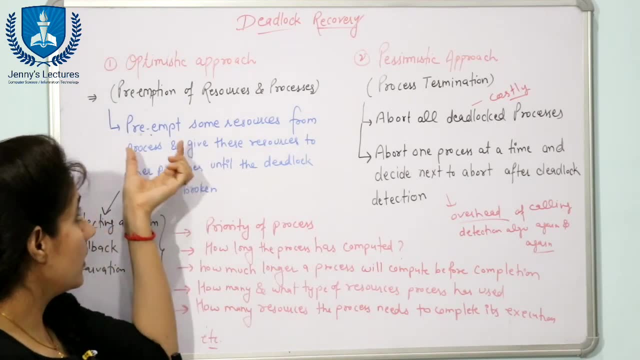 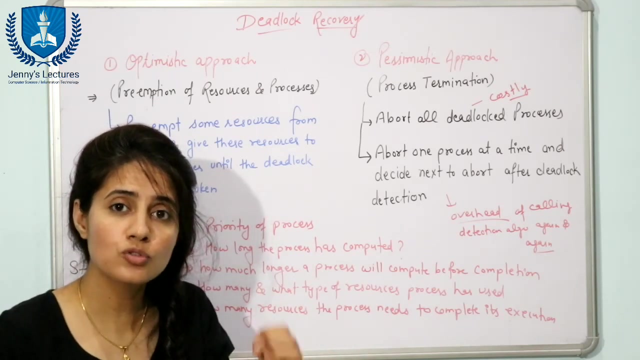 Now, what are these problems? So selecting a victim means you can say which resource or which process is to be preempted. Fine, Say here. here I am saying: preempt some resources from a process, from which process and which resource you will preempt. You have to select that one, So we will select that process. you can say: 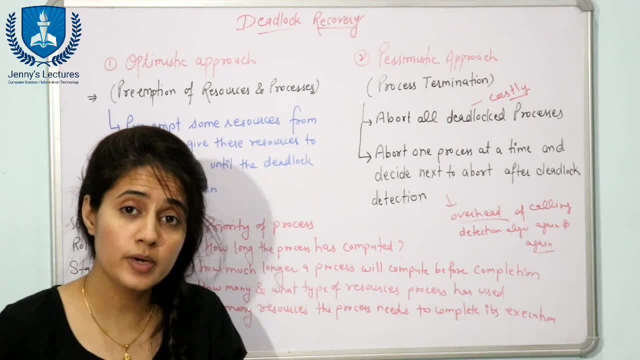 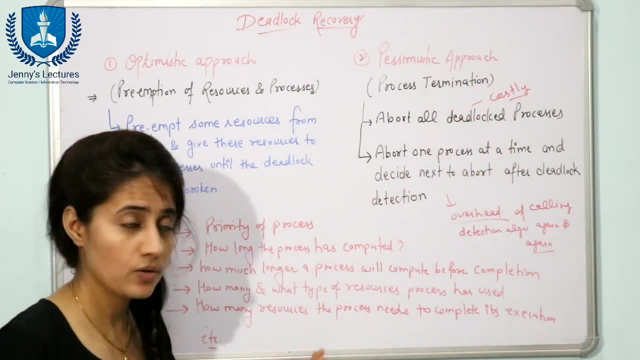 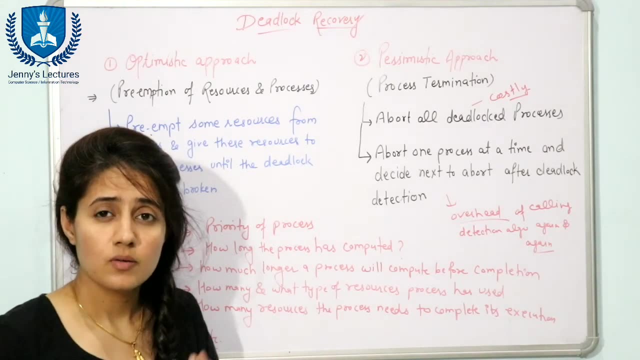 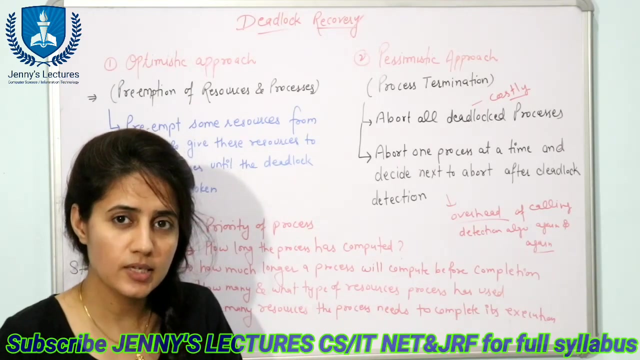 factors are there. See, here also we have considered these cost factors. Fine, when we are, we are selecting a process to kill, So here also these type of you know cost factors are there. like a number of resources are deadlocked, processes are holding, So here also some cost factors are there. 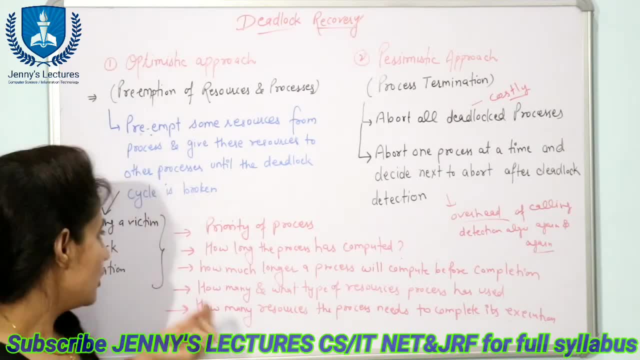 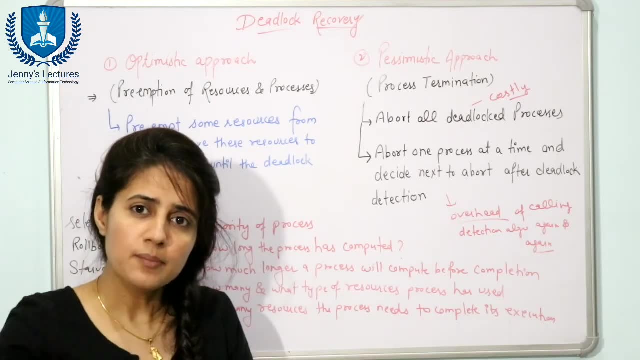 which is to be considered when we are selecting a victim process. Next fundai is this rollback. Now, what is this rollback? When you select a process and preempt it from stage two, if a product is to be preempted from stage, preempt resources from that process, then obviously that process cannot continue its normal execution. 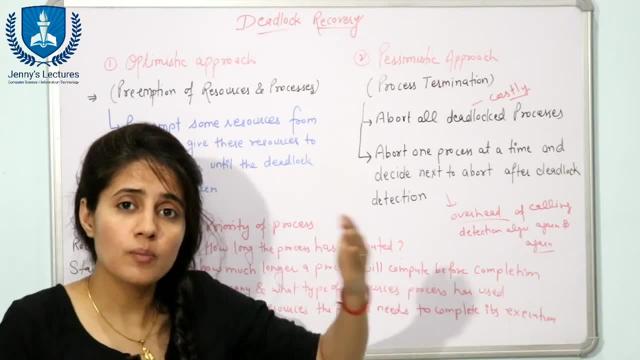 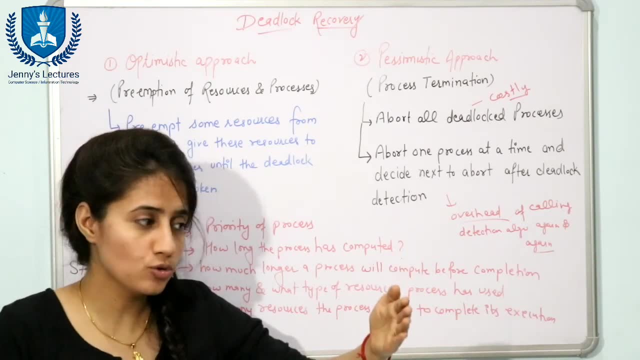 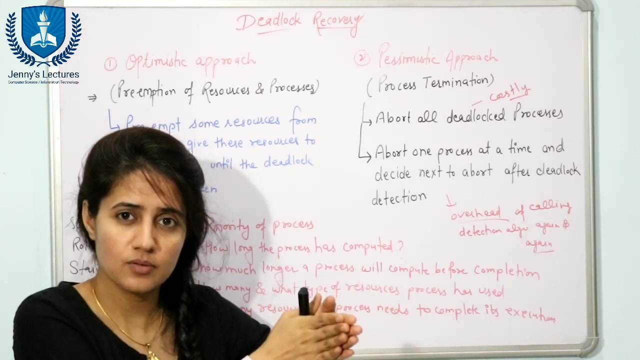 fine, then that process has to be rolled back to previous safe state and that process will start its execution from that safe state, only restart. you can say: restart its execution from that safe state, fine. or second thing is total rollback. you, you are selecting a, you have selected a. 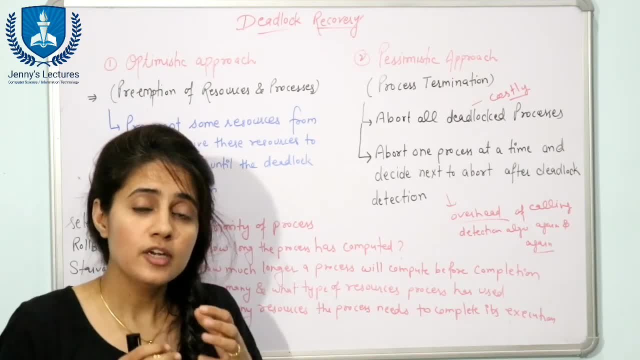 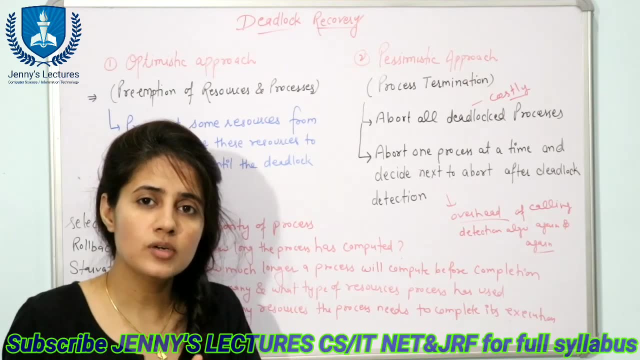 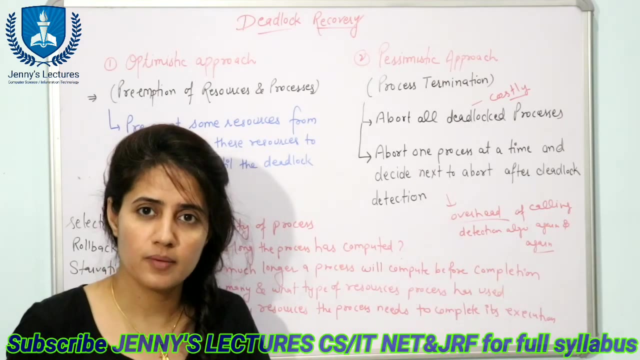 process, you have preempted some resources from that process, then you will do total rollback to that process. total rollback means you will, you can say about that process and that process will restart its execution from its initial point. that is total rollback, but it's better. it's better to. 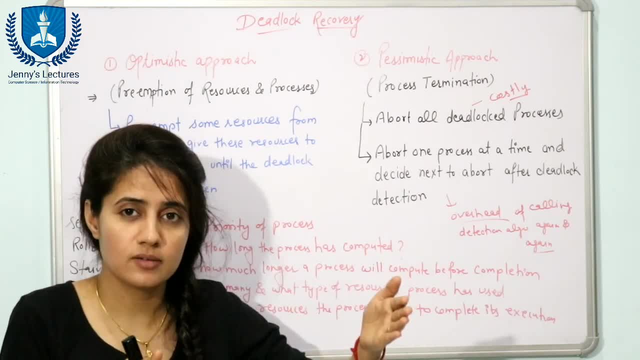 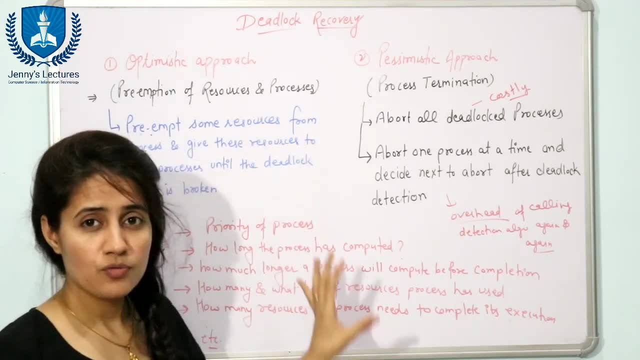 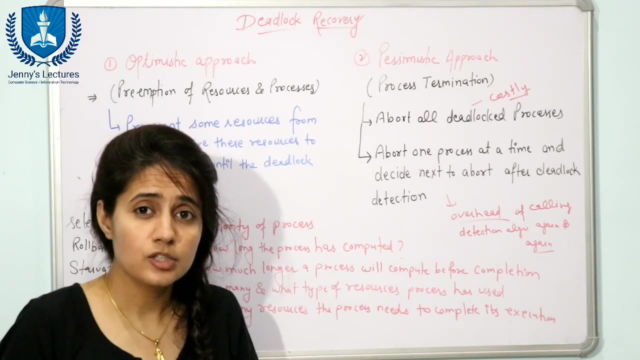 roll back a process to previous safe state. why so? let us take a real life example. suppose i am making this video fine and i have completed almost 50 percent of the lecture. maybe at last. at some point of time i told some wrong information, so i'll i'll reshoot the this video. i'll reshoot the video, obviously, from the point where i told: 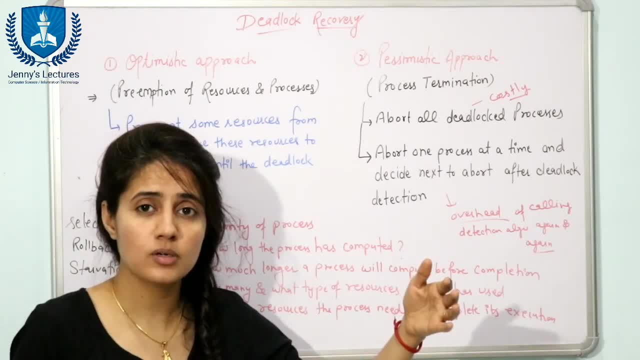 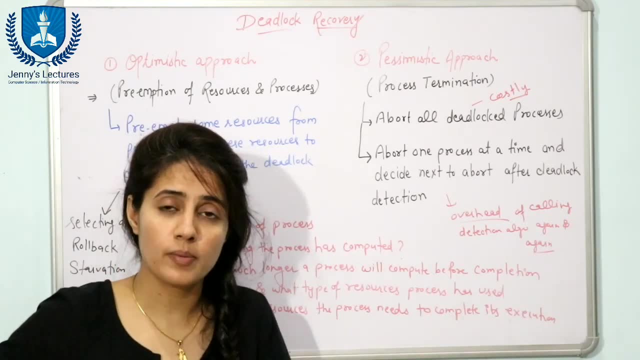 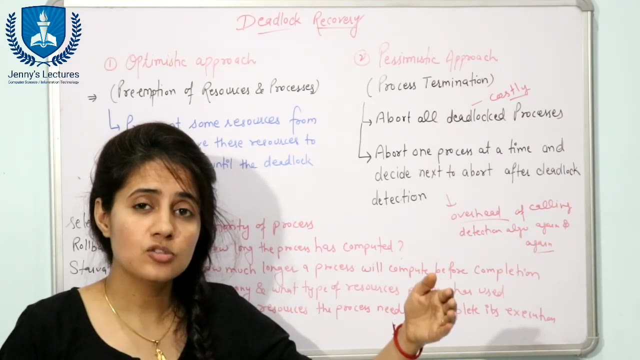 you that maybe some wrong information. i'll not reshoot the video, the complete video from starting. only if i'll reshoot the video from starting, it means total rollback and if i am reshooting the video from that point where i i told you the wrong information, then it. 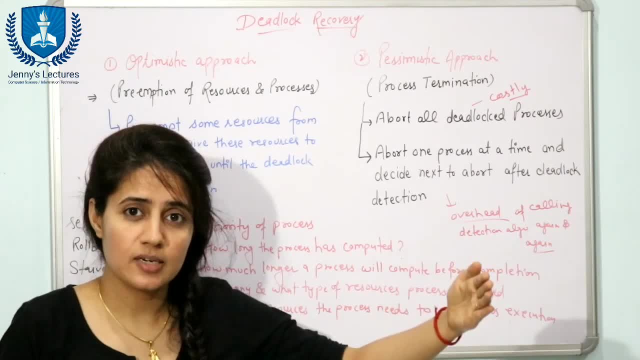 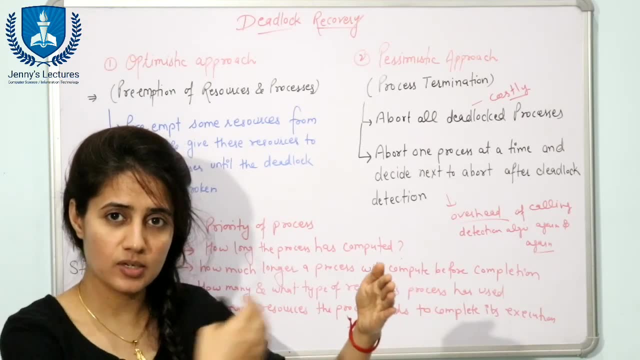 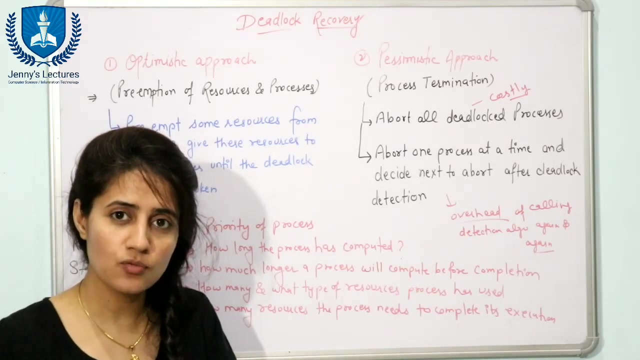 is known as rollback to some previous safe state. fine, so that is the rollback. funda in the process process will be rolled back to previous safe state and will restart its execution from that safe state. second thing is total rollback. the process which is selected as a victim is to. you can say: is to. 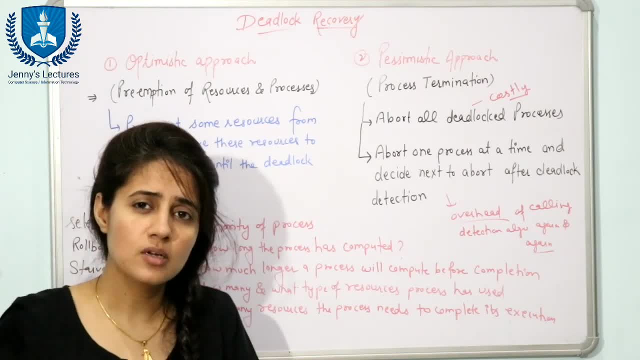 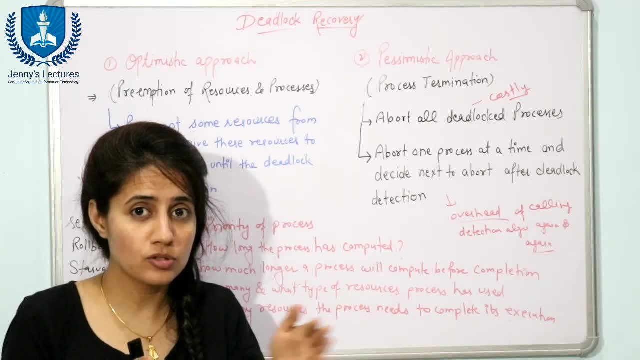 be aborted and that will restart it, its execution from its starting point only see it's better. what approach is better? it's better. that's how it works in some cases regarding the previous safe state safe state approach, better to roll back that process to previous safe state. but 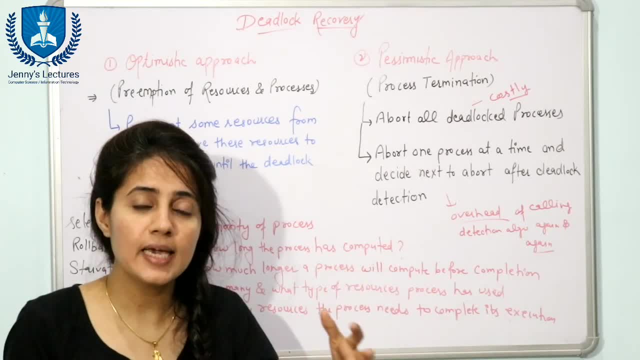 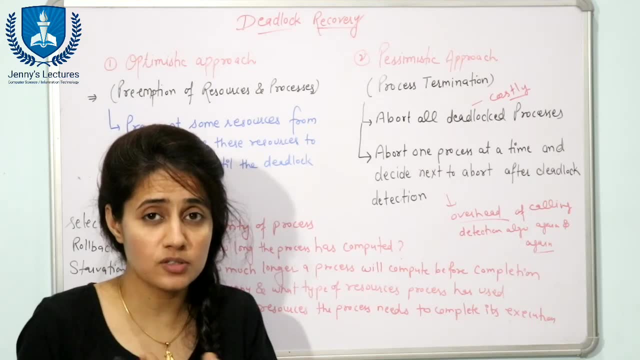 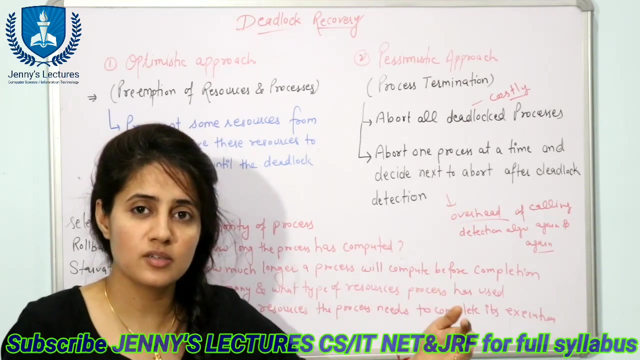 in that case? in that case system has to maintain the information of the state for all the running processes. obviously, if system has the information, till what point? what is the previous safe state? then only system can roll back to that safe state. now system can roll back that process to that safe state. so system 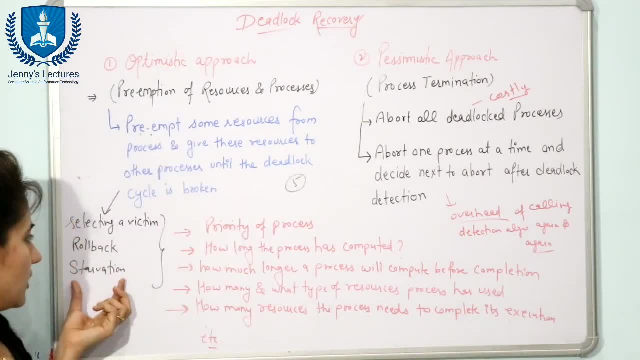 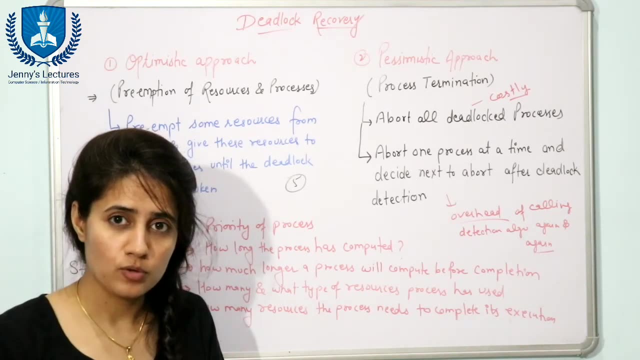 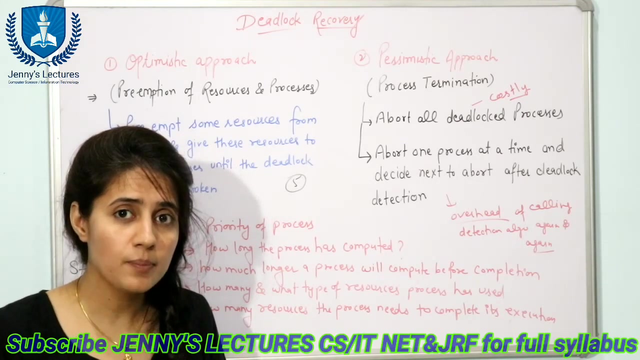 needs to maintain some extra information in this case. now, what is this starvation problem? see, in this case we are selecting a process and we are- we are preempting resources from that process. fine, but if again and again same process is selected for preemption, then what will happen then? starvation problem. 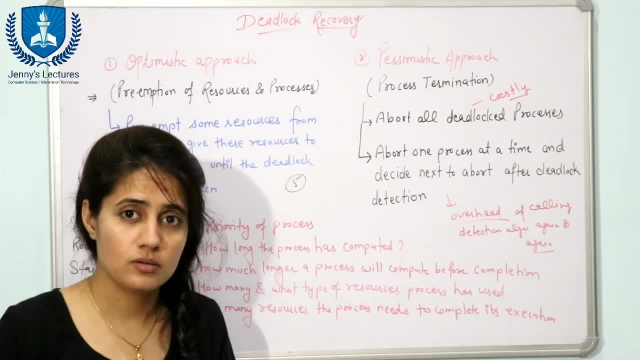 would be there for that process. that process will never complete its execution, will never be able to complete its execution. now, how to how to ensure that same process would not go through that system and then that process will not be selected as a victim again and again. so in for this system has to ensure that a particular 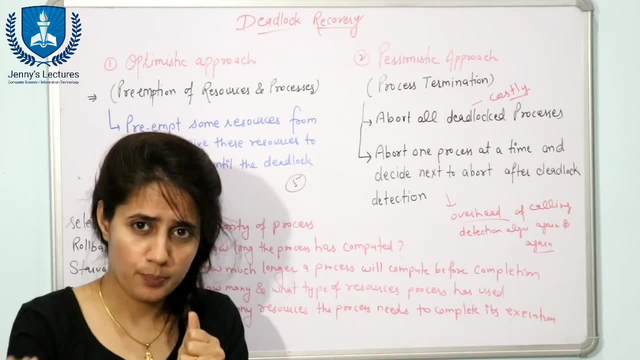 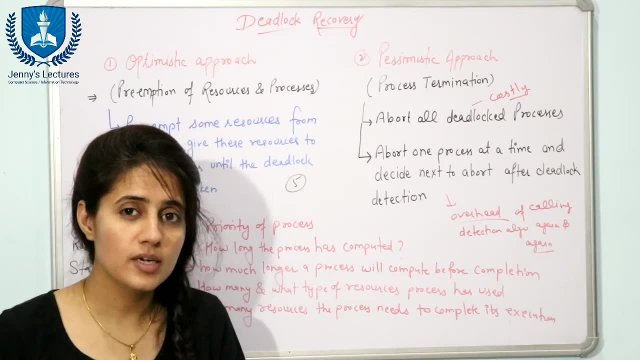 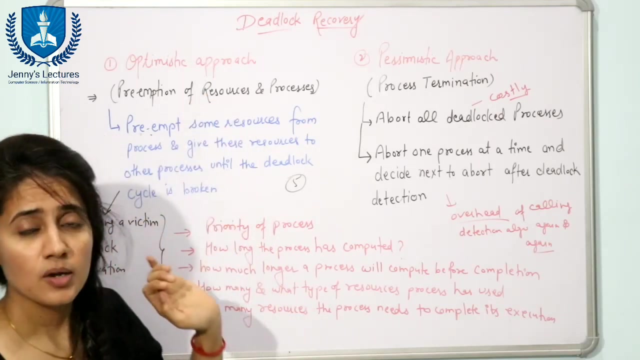 process can be, you know, picked as a victim for some finite number of time, and how this thing can be ensured, you can say in cost factor, many cost factors. we have discussed many cost factors. we will consider when we will select a process to preempt. so in those cost factors we can include.